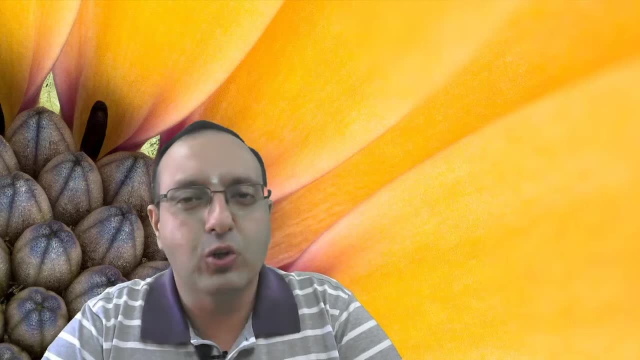 and poke holes in the scientific logic. So the criticism is about the second law of thermodynamics, which is a very well-recognized, well-proven law. So it's pretty much set in stone. There have been no exceptions to it And the second law of thermodynamics basically states that. 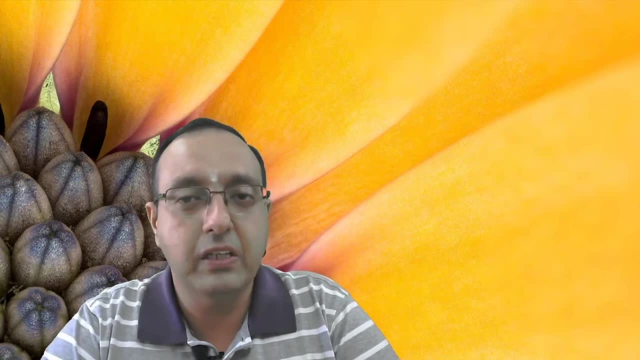 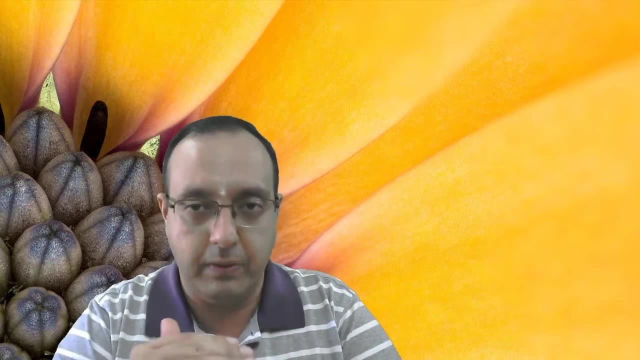 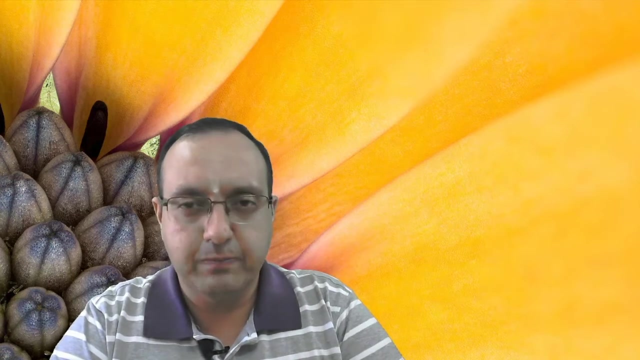 in all natural processes the entropy of the universe increases. So the focus is on the universe as well as the increase in entropy. Now I want to clarify a few things here first. So natural processes means any spontaneous process and universe here does not mean the. 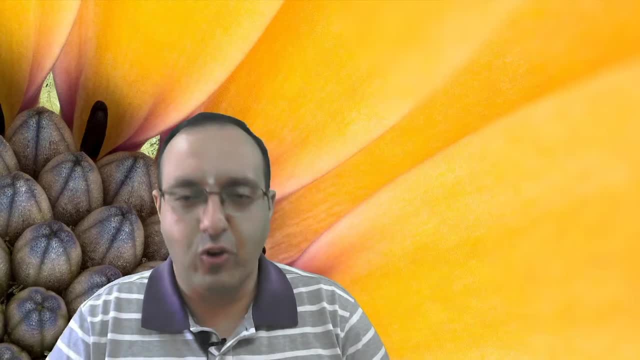 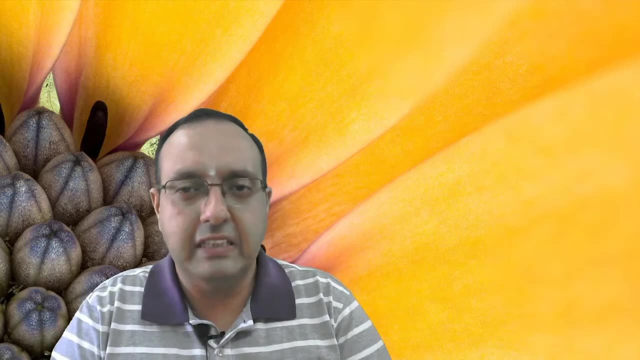 whole universe, the Milky Way and the Andromeda galaxy. no, we are not talking about that. We are only talking about a system that we are studying and its surroundings. So, for example, if we take a kettle filled with warm water, along with the room where it is kept, 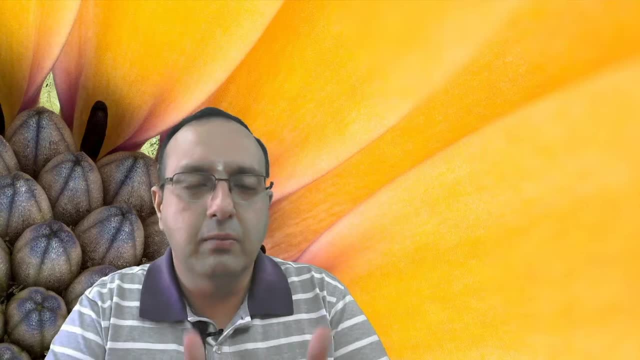 that is the universe that we are creating. So, at the same time, if we put the heat in, we can actually start cooking and that is the result of the process. So, for example, to talk about, and similarly for human body or any animal body or plant body, any organism. 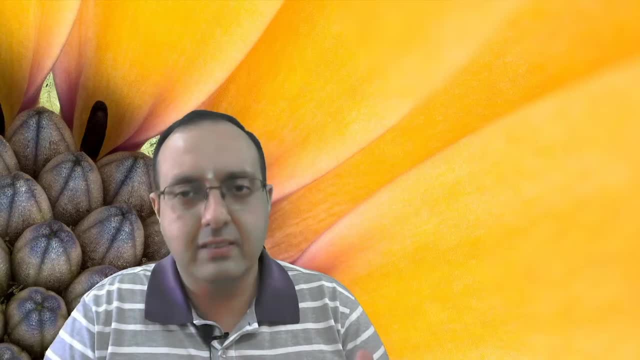 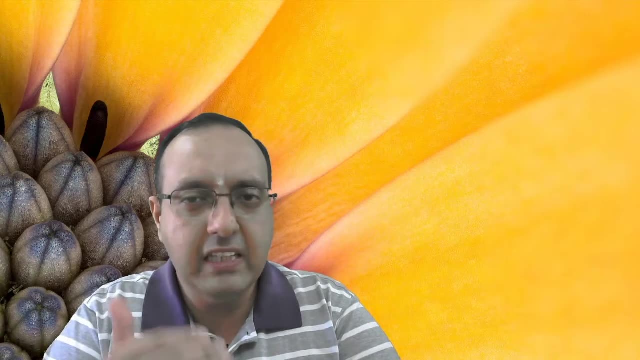 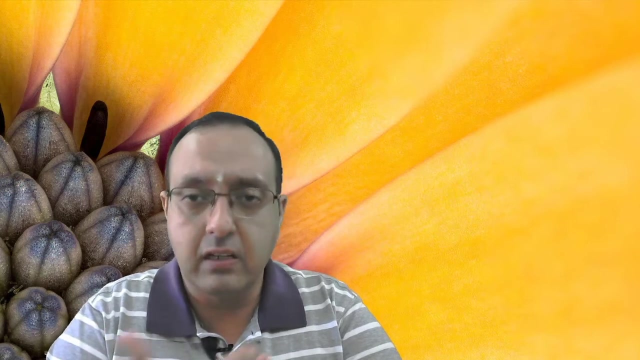 the immediate surroundings of that organism, plus that organism is the universe. so the second law of thermodynamics says that if, in order for any spontaneous process to happen- and in case it happens, of course it happens- the entropy of the universe increases the entropy of the total system, 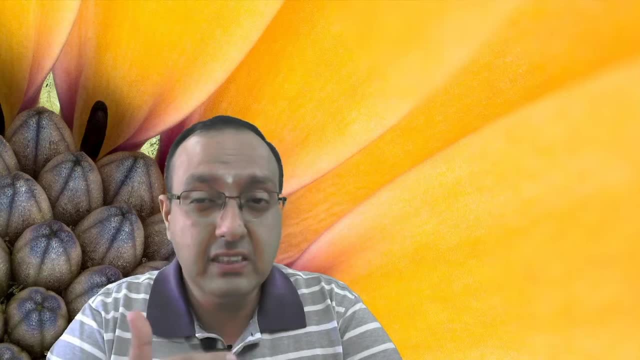 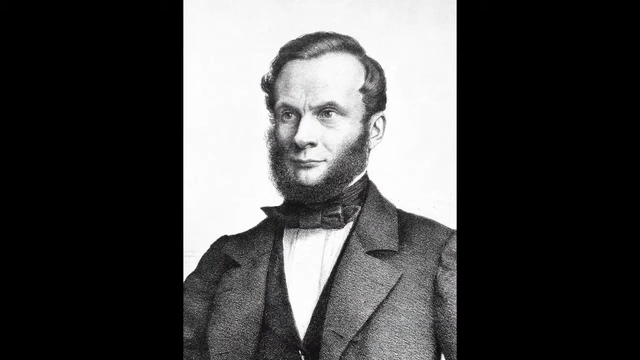 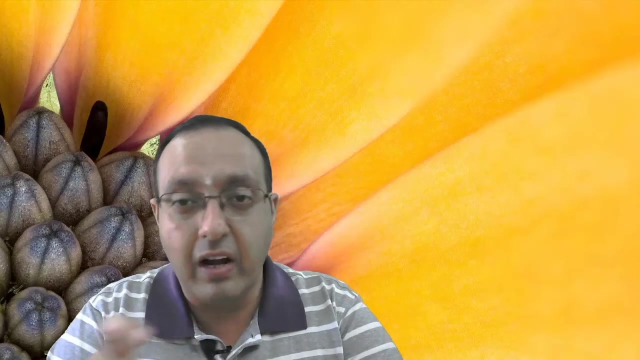 plus surroundings increases. now this seems, you know, a little bit counterintuitive. the idea was first proposed by rudolph clausius in 1865, and entropy, as he defined, was referring to the disorderness or randomness of the system. so, for example, if we take, for example, a tiny 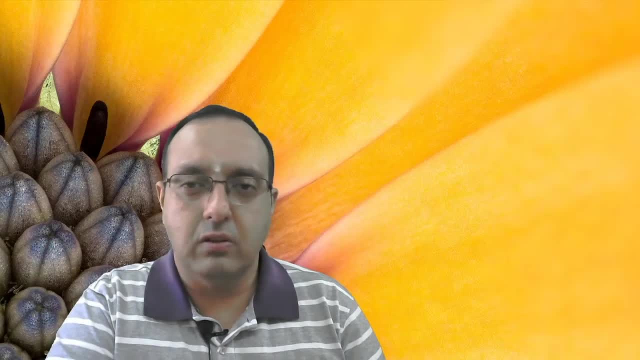 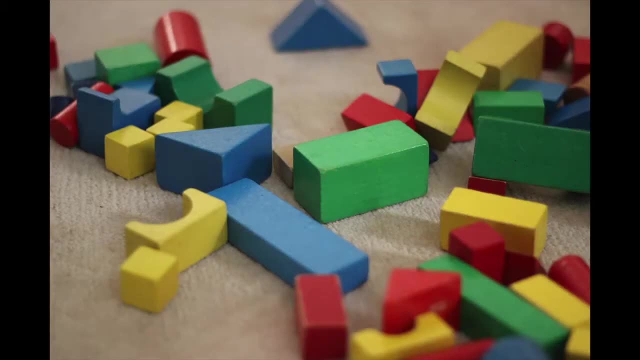 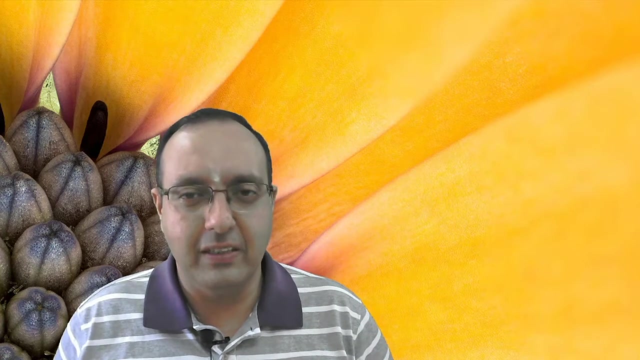 well-organized room. that is kind of a room you or system you can consider with low entropy. and, on the other hand, if we consider a cluttered room, disordered room, right, like for example you might find in dorm rooms or hostels, right, those are examples of high entropy surroundings. so 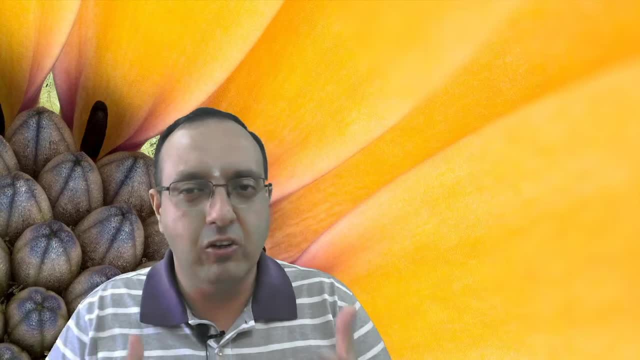 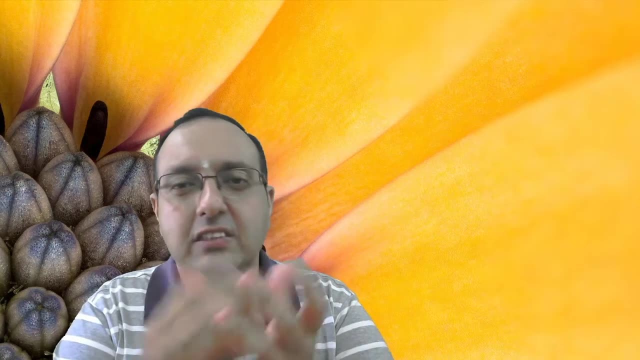 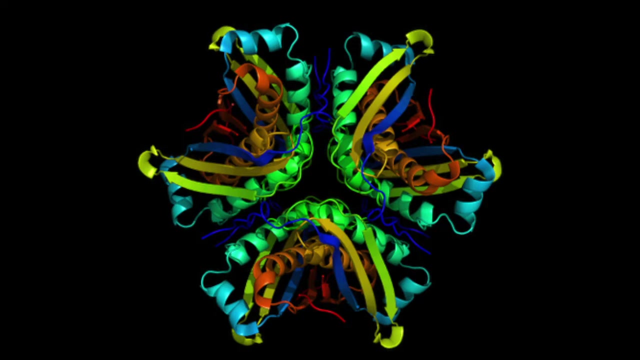 if you look at the human system or organisms, living organisms, it does not seem like they are following the second law of thermodynamics. because if you look at even the simplest organisms, for example viruses, bacteria, even our protein molecules, dna molecules, they are highly structured right dna molecules are so long they have this compact organization. 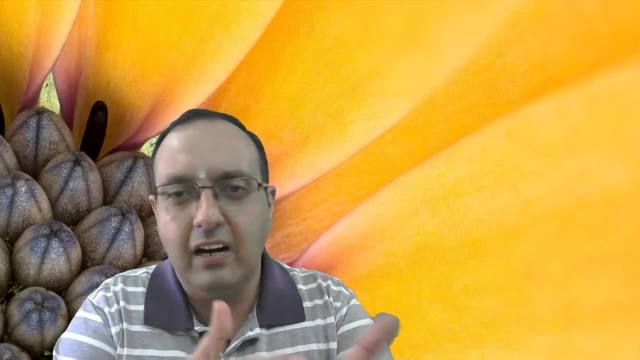 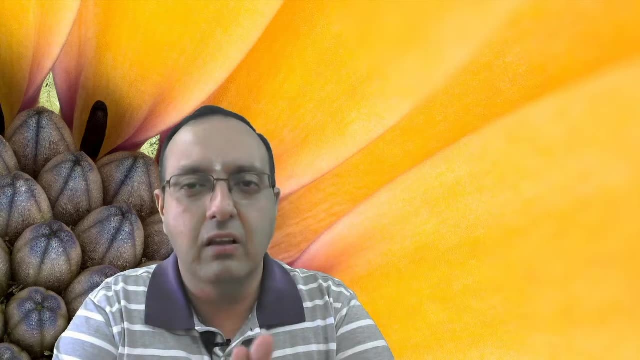 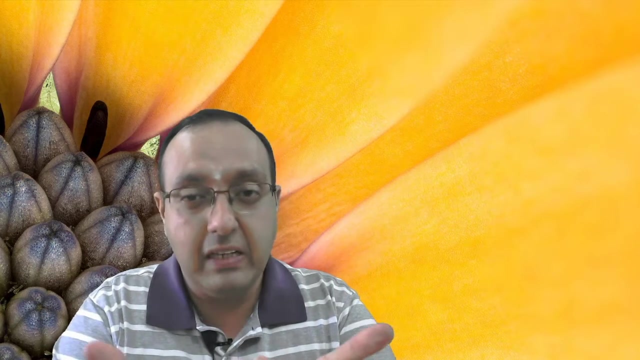 every cell has a nucleus, golgi complex, er, ribosomes, all the stuff which is very, very tightly regulated, and there are intricate structures forming in living organisms all the time. so do living organisms violate the second law of thermodynamics. that's what many science deniers and that's what 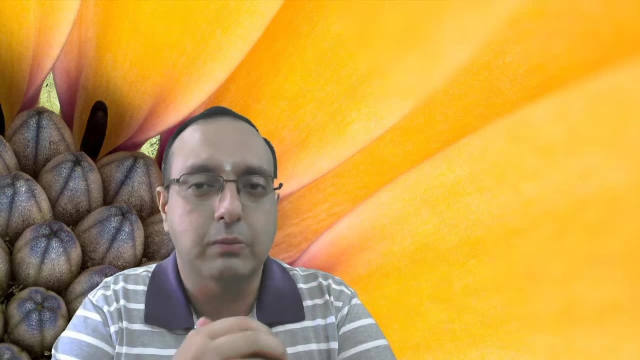 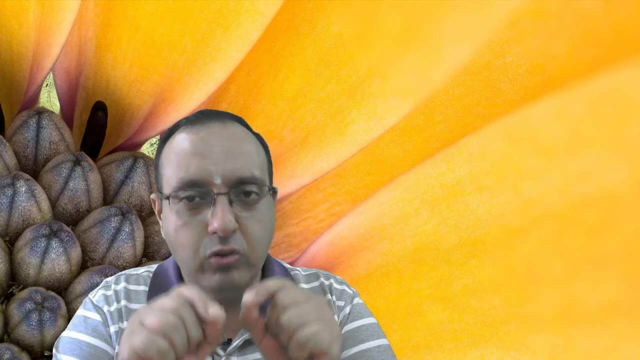 many, you know, people who are not very familiar with these concepts of biochemistry, seem to be not familiar with the concepts of biochemistry, seem to be not familiar with the concepts of biochemistry to think. but actually that's not true, because the emphasis, if you think about it, it's on the 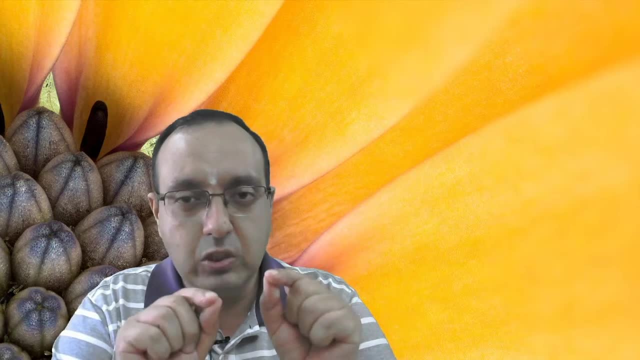 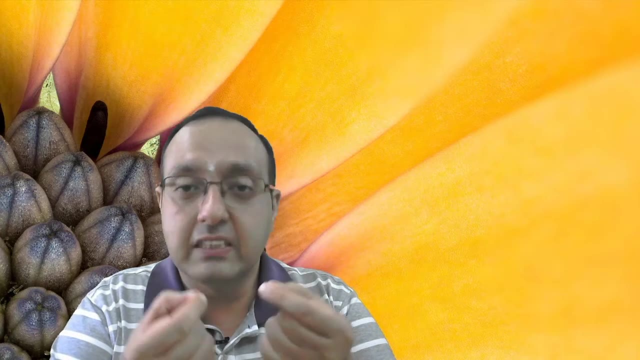 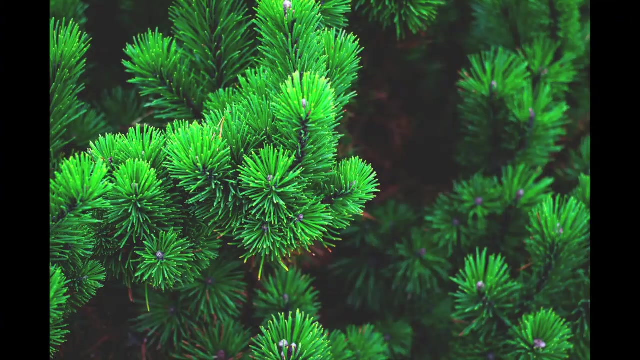 universe, which is the system plus surroundings. so if the total entropy of system plus surroundings increases, there is no problem. and that's what actually living organisms do. they take in food materials, whether it be sunlight or inorganic nutrients, in case of bacteria or plants, or, for example, other organisms, in case of. 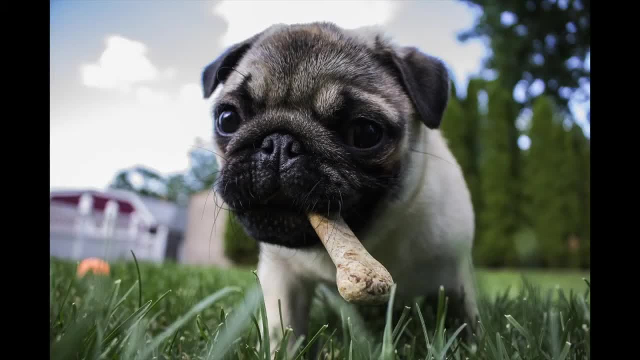 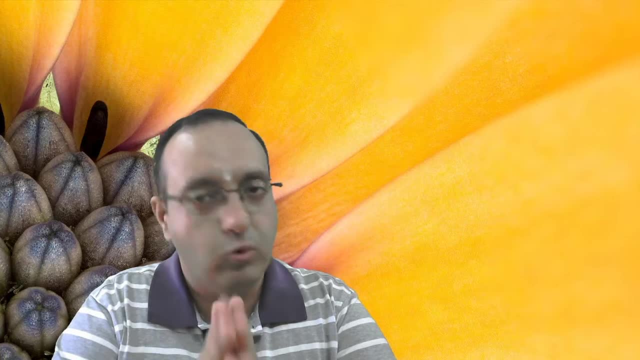 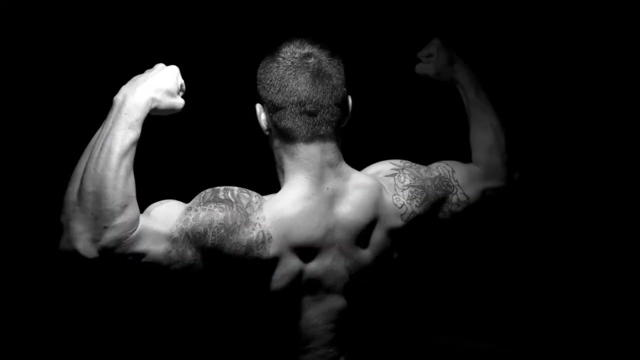 herbivores, carnivores, omnivores, like us. we take food molecules. we take, you know, these nutrients and we catabolize them, we process them through our metabolism and what we do is we use them to make our own tissues, our own molecules. so we use them, for example, to produce new red blood cells. 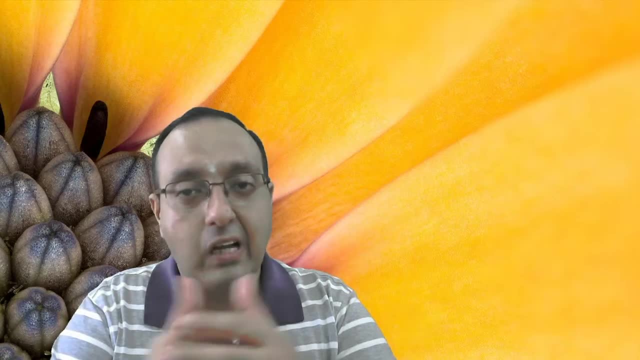 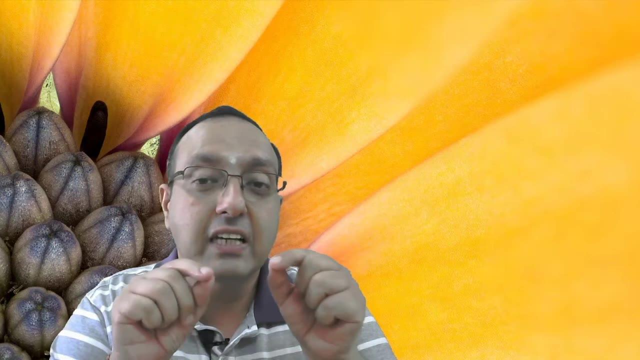 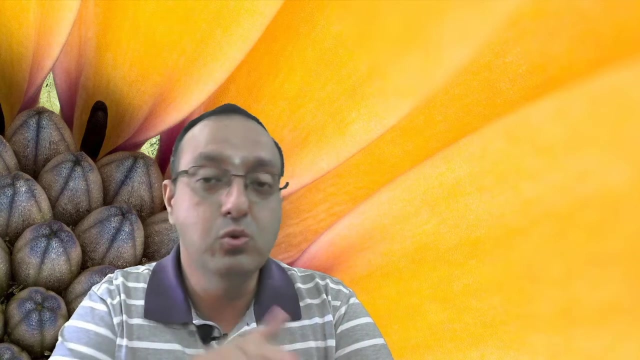 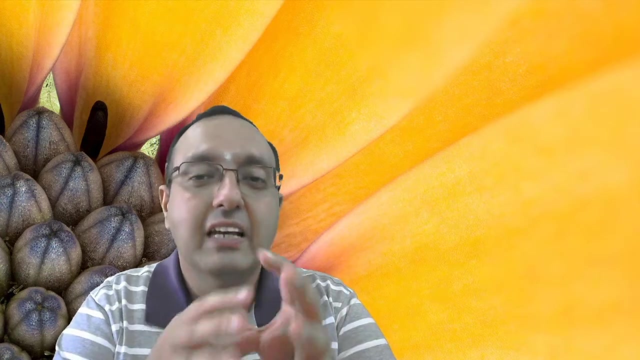 new muscles, new tissues, new skin, you know, new gut lining, everything right. but here is where the uh part is, because this is where entropy is decreasing. of course it leads to more order. you know a huge DNA molecule. as compared to just single nucleotides, it's highly ordered. the solution is increased. 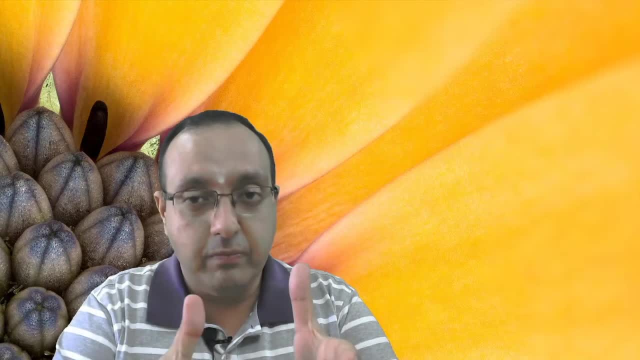 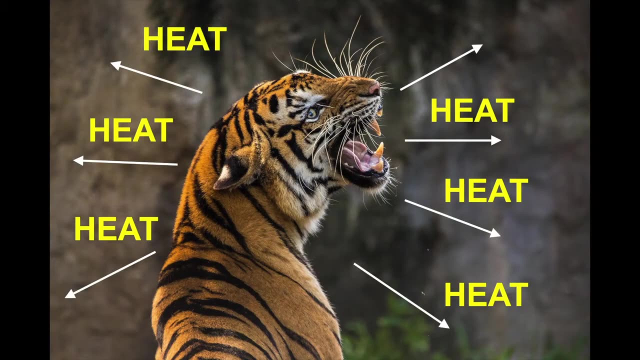 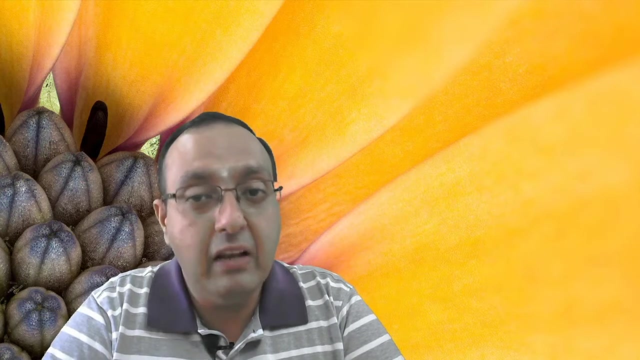 entropy outside. so here is the solution to that problem. living organisms produce a lot of heat, random heat, which is unusable- it does not apply for the, for example, gibbs- free energy which is available to do useful work. and they also produce a lot of simple waste compounds- urea, ammonia, uric acid, urine poop.